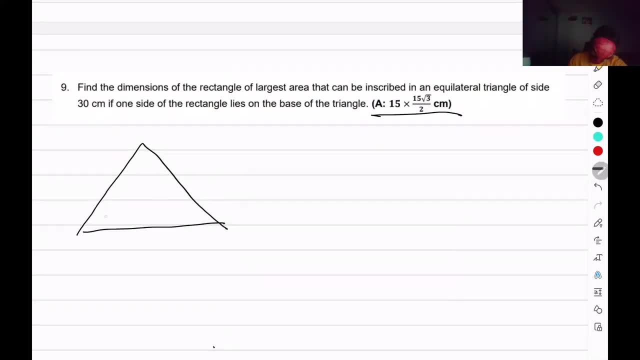 So here's an equilateral triangle and the rectangle is inscribed inside it where it is touching the base. So in these inscribed questions I like to draw it on a grid. So we know one side is 30 cm. 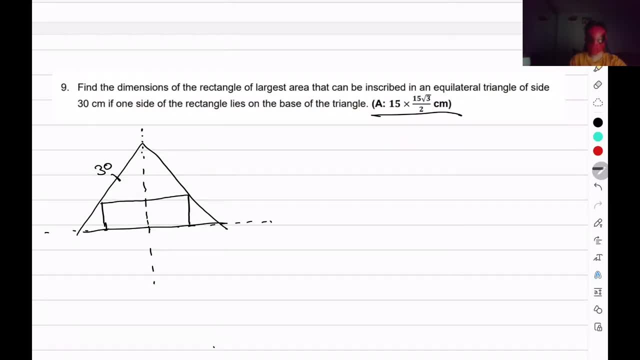 So I drew this. the y-axis is bisecting this triangle, So this point right here is 15.. This point right here we can find in an equilateral triangle. all angles are 60 degrees, So we can find the height using Pythagorean theorem. 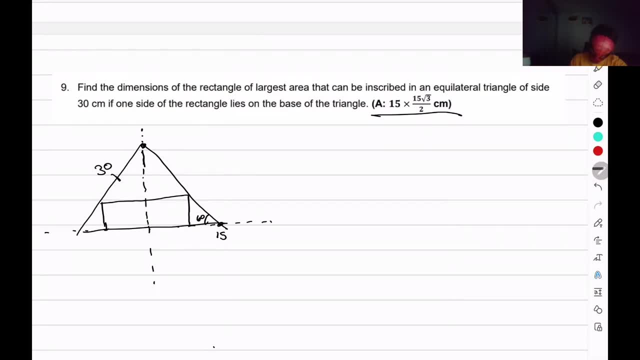 Sorry, not Pythagorean theorem, but using trigonometry. So height is equal to 30 sin theta, Which is equal to 15 root 3., 3., 3., 3., 3., 3. 3.. 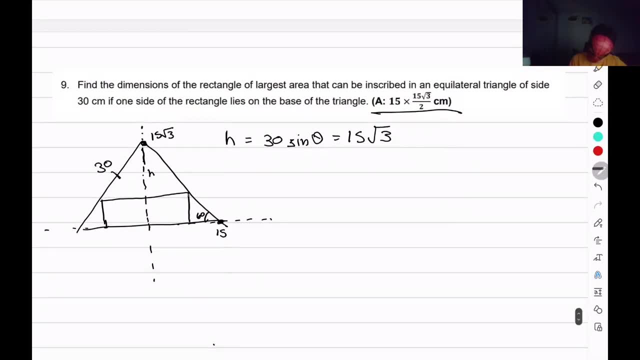 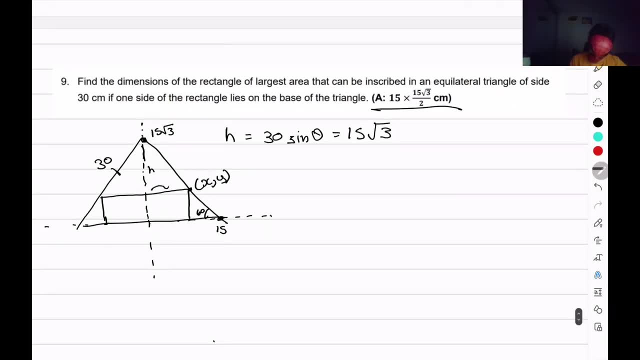 Now why did I do this? The x basically represents the distance from this y-axis to here is x, And the same distance from this y-axis to here is also x. So that represents the length. So the length is equal to 2x. 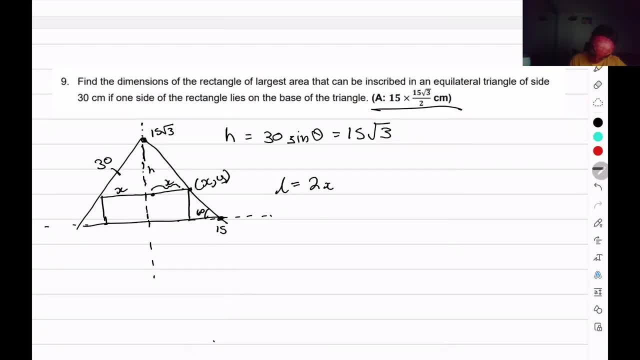 Now what does the y represent? The y represents the height from here to here, so basically the width of this rectangle. so the width is equal to the y. now, what is y in terms of x? because we need only we need one variable to optimize, right. so the y is basically.